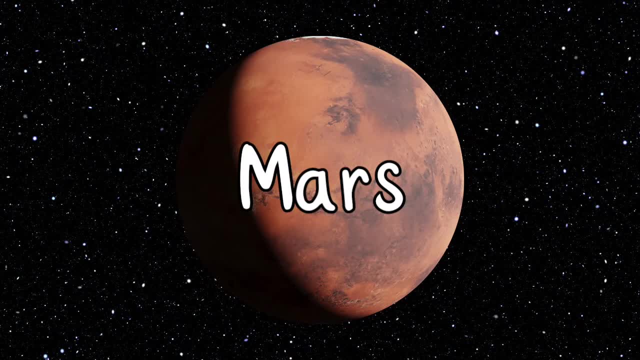 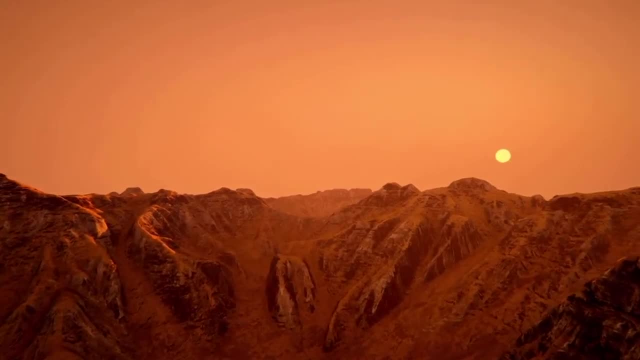 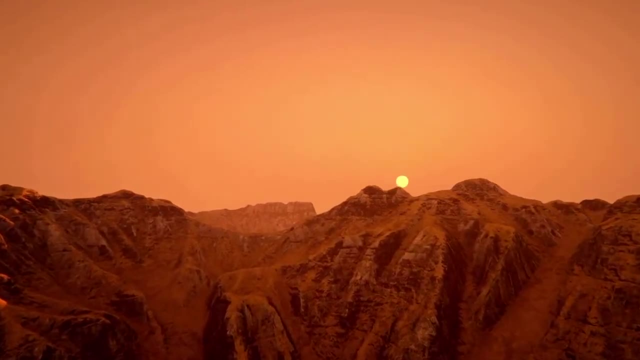 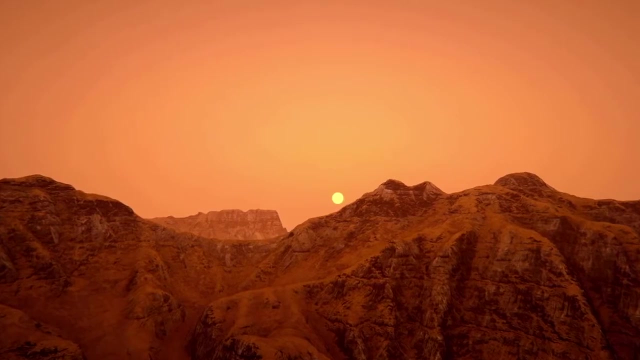 Mars. Mars is the fourth planet from the Sun and the second smallest planet in the Solar System, Right after Mercury. its orbit around the Sun takes 687 Earth days. 24 hours and 37 minutes is a day on Mars, which is 37 minutes longer than a day on earth, to be exact. fun fact, mars was once a watery planet. 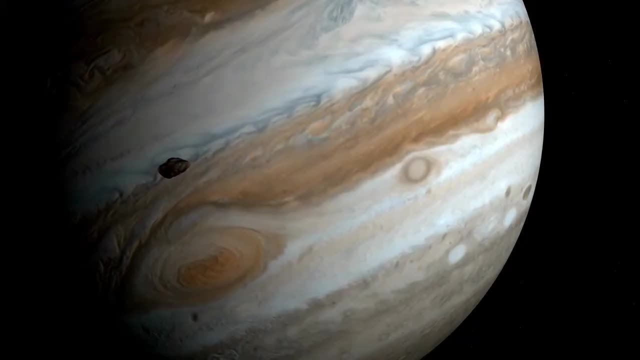 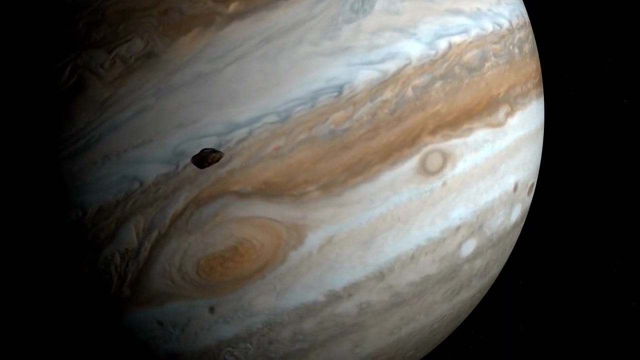 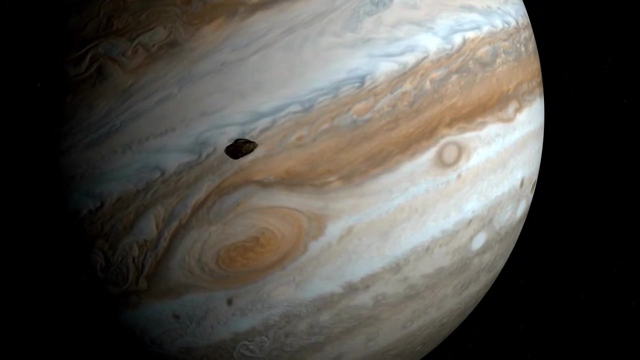 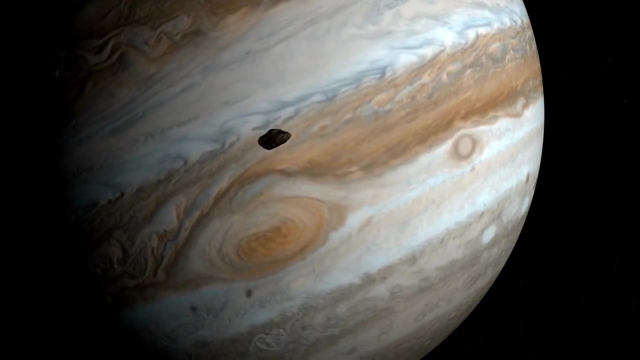 jupiter. jupiter is the fifth planet from the sun and the largest in the solar system. its orbit around the sun takes 12 earth years. 9 hours and 56 minutes is a day on jupiter. fun fact: jupiter is made mostly of gas, with more than double the mass of all the other planets combined. 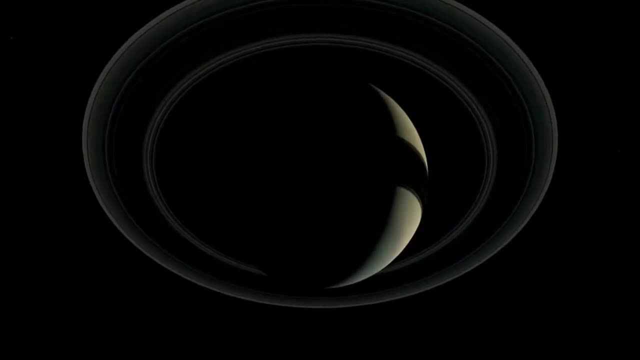 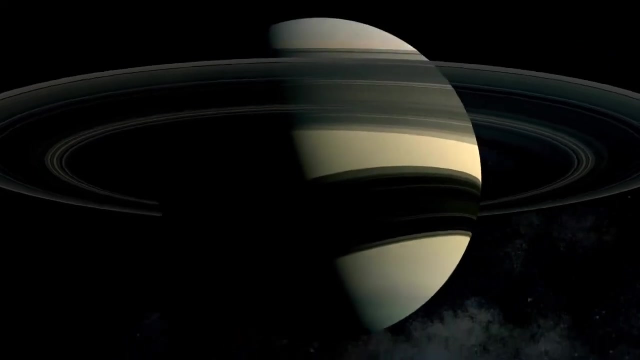 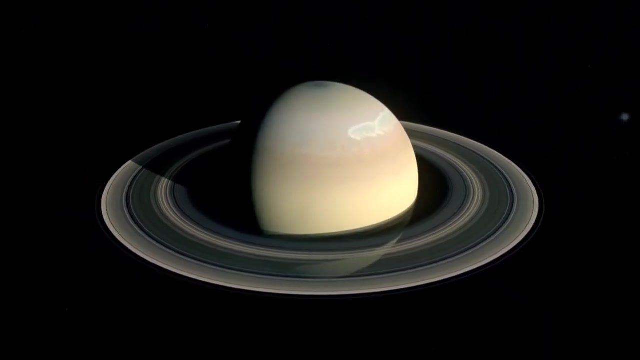 saturn. saturn is the sixth planet from the sun and the second largest in the solar system after jupiter. its orbit around the sun takes 84 earth years. 17 hours and 14 minutes is a day on saturn. fun fact because saturn is made mostly of gas. 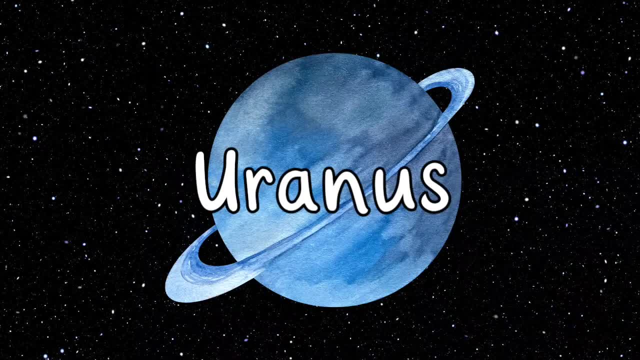 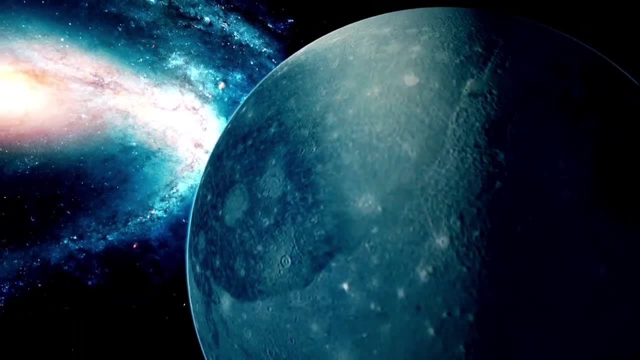 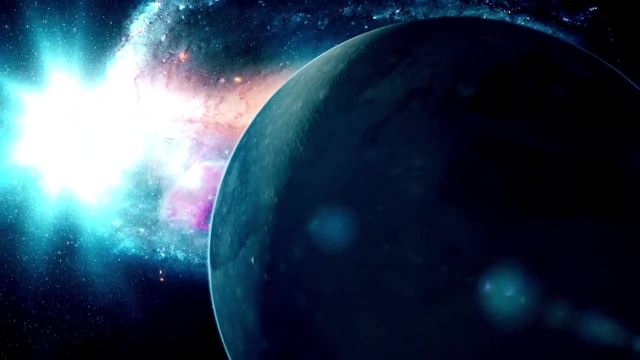 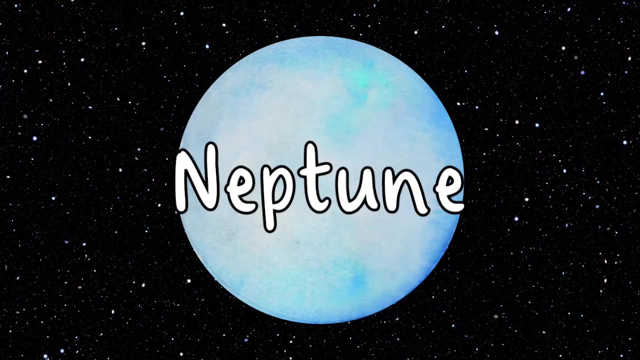 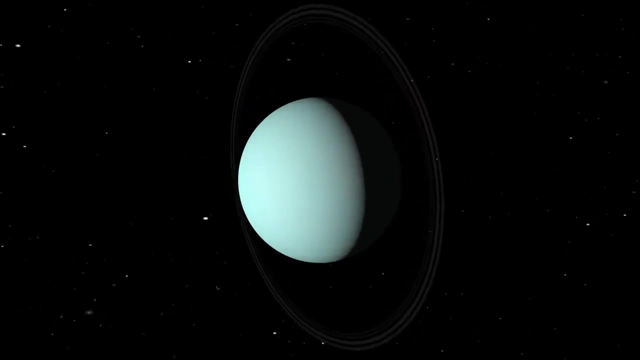 this planet could float in water uranus. uranus is the seventh planet from the sun. its orbit around the sun takes 29 earth years. 10 hours and 42 minutes is a day on uranus. fun fact: uranus rotates on its side neptune. neptune is the eighth and farthest known solar planet from the sun. 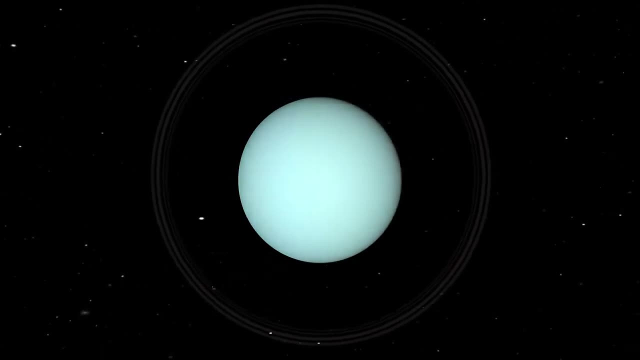 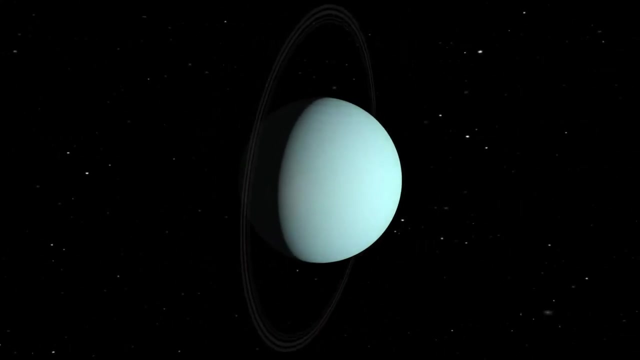 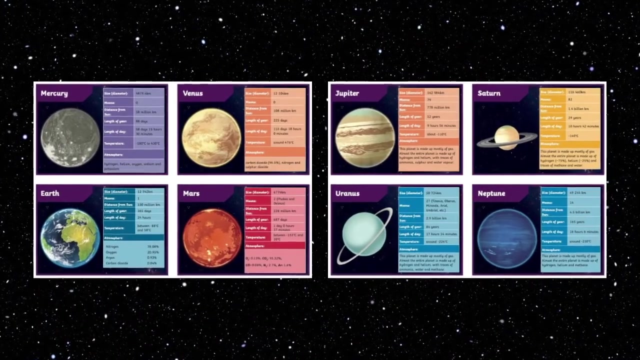 its orbit around the sun takes 165 earth years. 16 hours and 6 minutes is a day on neptune. fun fact: Neptune is the coldest planet in the solar system, Just like this Planets of the Solar System. fax card Twinkl has lots of resources for Space Day planets and the solar system. 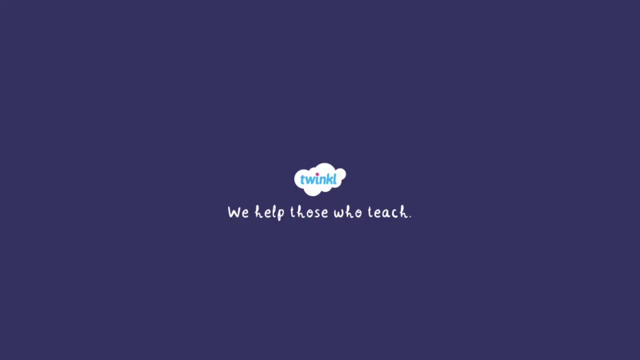 For more resources, check the description below.